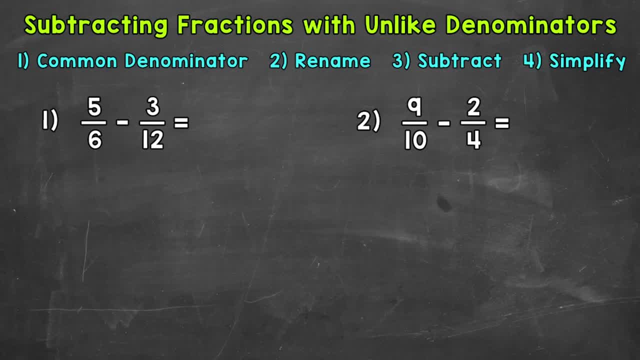 In this video, I'm going to cover how to subtract fractions with unlike denominators. So let's jump into our examples, starting with number 1, where we have 5 sixths minus 3 twelfths. Now when we subtract fractions, we need a common denominator, just like when we add fractions. For number 1, we have a 6 and a 12, so we don't have a common denominator to start with, so we can't subtract quite yet. The first thing that we need to do is find a common denominator, and we can do that by finding the least common multiple between our denominators. We want the least because smaller numbers in value are generally easier to work with, and this will help cut down on simplifying in the end once we get to our answer. As far as why we need a common denominator, that's a topic for another video. I'll drop that link down in the description. Now as you're looking at a subtraction problem involving fractions with unlike denominators, you may recognize the least common multiple between denominators right away. 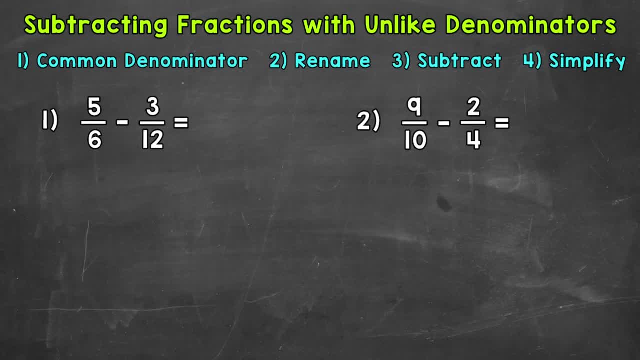 But if not, you can always write out your lists of multiples in order to find it. So let's start by writing some multiples of both 6 and 12, and see if we can find that. 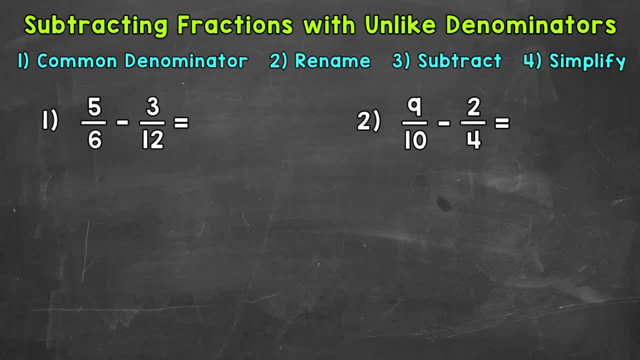 We'll start with 6, so I'm going to come to the bottom of the screen where I have some extra room to write out these lists, and we'll start with 6. So I would suggest writing out 4 or 5 multiples for each denominator, and see if you can find that least common multiple. 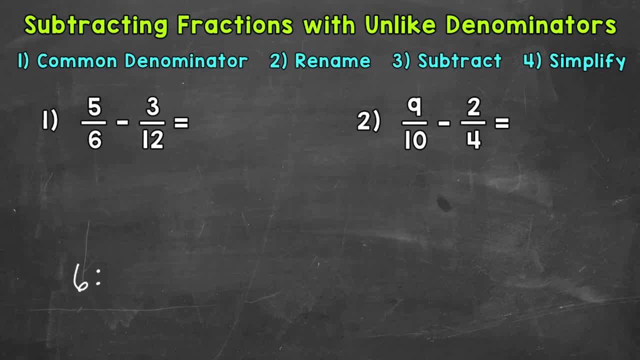 If not, you can always extend the lists until you find that least common multiple. So if 4 or 5 multiples don't work, and you don't see any common multiples, you can always write out your lists until you find that least common multiple. 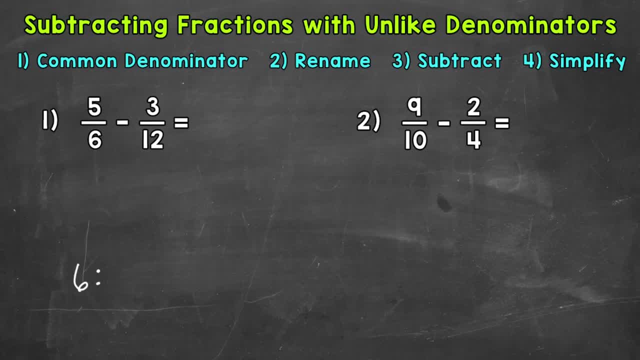 Extend those lists. So the first 4 multiples of 6 are 6, 12, 18, 24. Now we'll do 12. So the first multiple of 12 is 12. 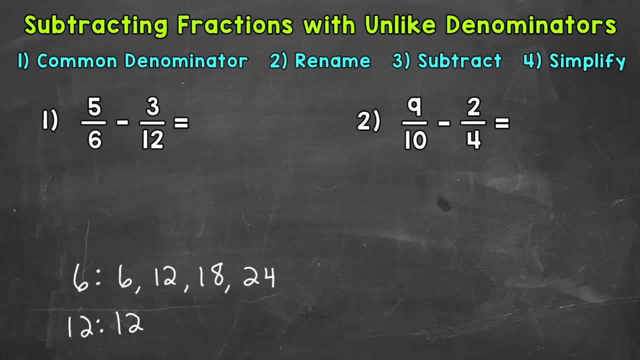 Now no need to go on if you find that least common multiple, because if you look, we have a least common multiple of 12. So we are ready to move to the next step. Which is rename. 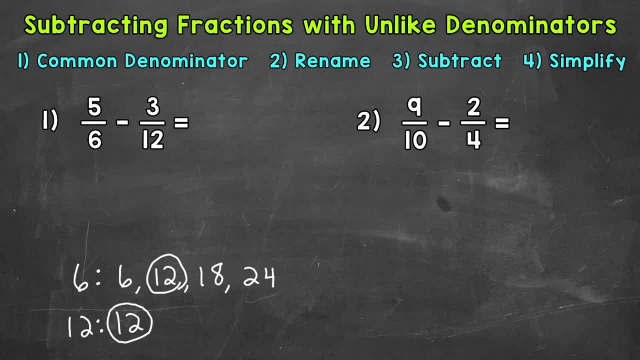 So 12 is going to be our common denominator. I'm going to come back up to the original problem, underneath, and start to write the renamed fractions with that common denominator of 12. So underneath, I'll start these fractions with that common denominator of 12. 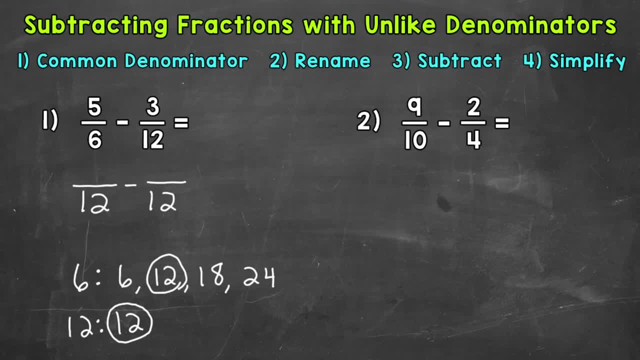 And now we're going to rename. We'll start with 5 sixths. 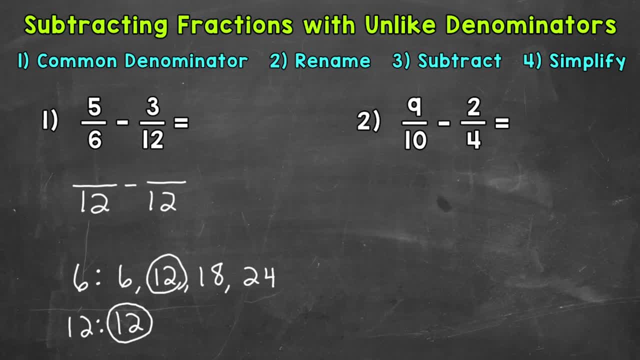 So we're going to rename that fraction with an equivalent fraction with the denominator. 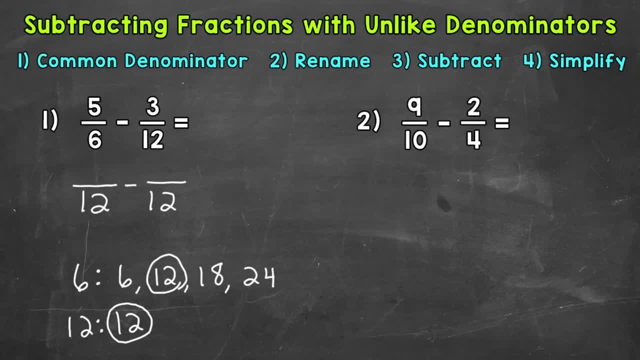 So we need to think, how do we get the denominator of 6 to equal the denominator of 12? 6 times what equals 12? Well, we know that 6 times 2 equals 12. So whatever we do to the denominator, the bottom number, we have to do to the numerator, the top number, in order to keep this fraction equivalent. We don't want to change the value of the problem at all. So we need to think, how do we get the denominator of 6 to equal the denominator of 12? So we need to do 5 times 2 to get the renamed numerator. 5 times 2 is 10. 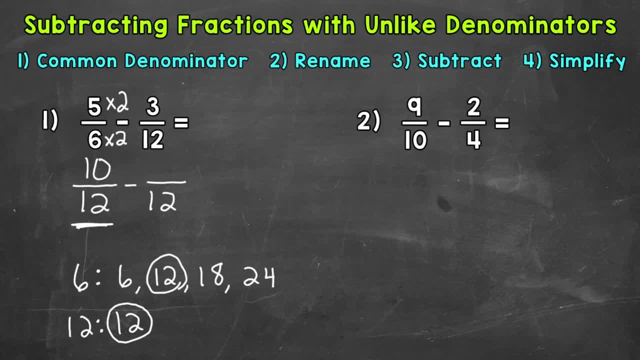 So 10 twelfths is equivalent to 5 sixths. So we renamed with that denominator of 12. Now we need to do 3 twelfths. Well, 3 twelfths already has a denominator of 12. So we don't need to rename. We can just bring the 3 down. Once we rename, we can subtract. When we subtract fractions, we subtract the numerators. So 10 minus 3 is 7. 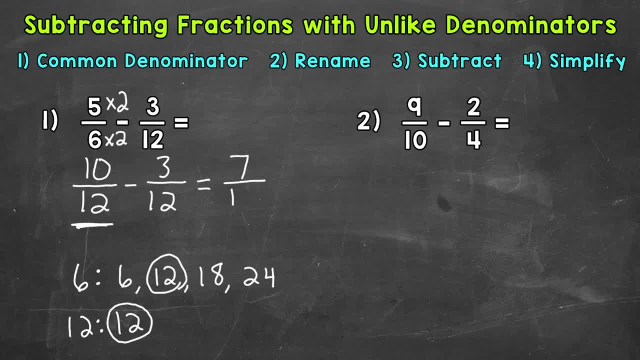 And then we keep the denominator of 12 the same. 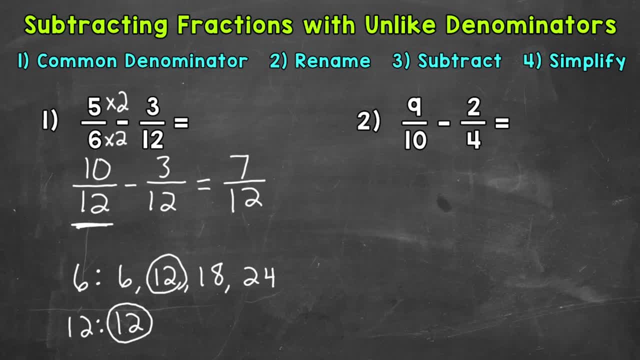 So 7 twelfths is our answer. Now always look to simplify. So can we simplify 7 twelfths? Well, 7 twelfths is in simplest form. The only common factor between 7 and 12 is 1. So we can't break this down. We can't go any further as far as simplifying goes. So our final simplified answer, 7 twelfths. 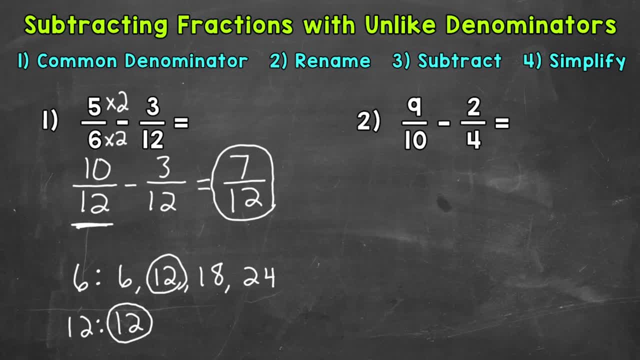 Let's try another one and move on to number 2 where we have 9 tenths minus 2 fourths. So the first thing that we need to do, find a common denominator. So we need that least common multiple between 10 and 4. And that's going to be our common denominator. Let's go down to the bottom and write out some multiples. So we'll start with 10 and we'll write out 4 multiples to start with. So 10, 20, 30, 40. Now let's write out 4 multiples of 4 and see if we have a least common multiple. So 4, 8, 12, 16. 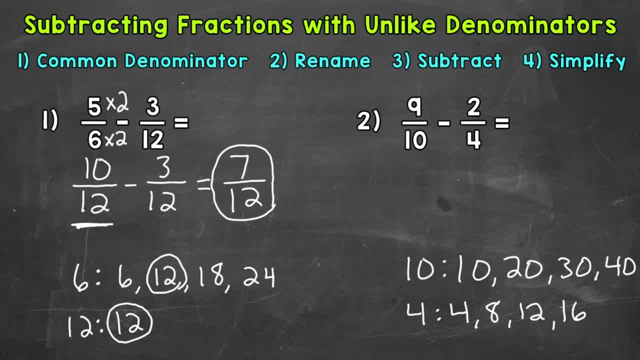 So writing out 4 multiples for each, we don't have a match. 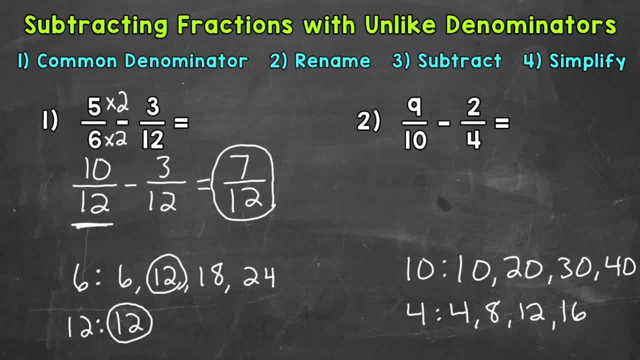 So we need to extend our list. Now the multiples of 10, we are already at 40. And the multiples of 4, we're only at 16. So let's extend that one. And the next multiple of 4 is 20. And that's going to give us a common multiple and specifically the least common multiple. So we're going to use 20 for our common denominator. Let's go back up to the original problem underneath and rename with that common denominator of 4. 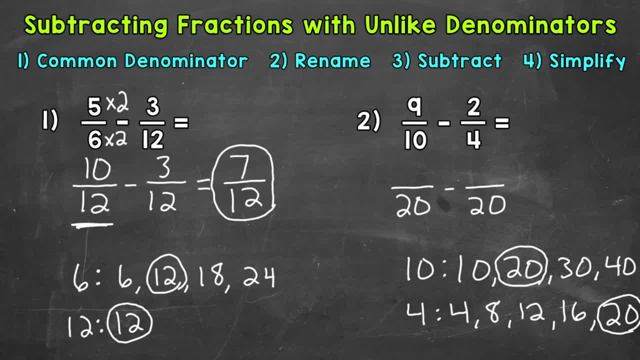 20. We'll start with 9 tenths. So how do we get that denominator of 10 to equal 20? Well, 10 times 2 is 20. And whatever we do to the denominator, we have to do to the numerator in order to keep this equivalent. So 9 times 2 gives us 18 for our renamed numerator. So 18 twentieths is equivalent to 9 tenths. We just have that common denominator of 20 now. Now we need to do 2 fourths. So how do we get 4 to equal 20? 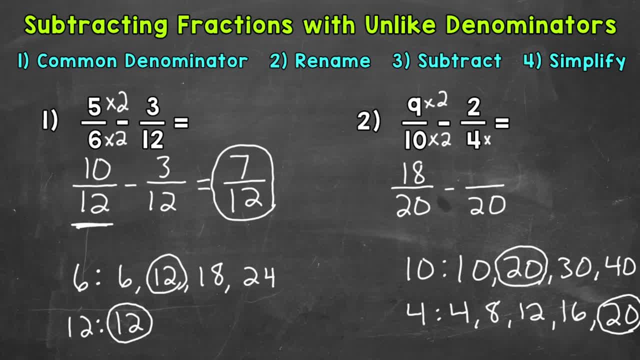 Well, we know 4 times 5 equals 20. So 4 times 5 equals 20.